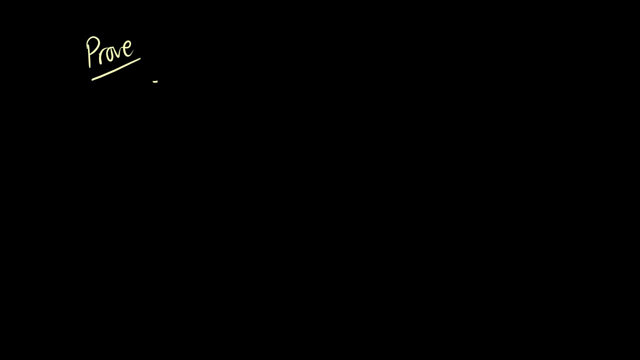 camera, because it's the exact same steps. but prove that if 7 divides 4a, then 7 divides a. exactly the same steps. uh, do that on your own, put it in the comments and i'll tell you if it's right or not. okay, so here's the second one. prove that every odd step is equal to 7 divided by 4a. 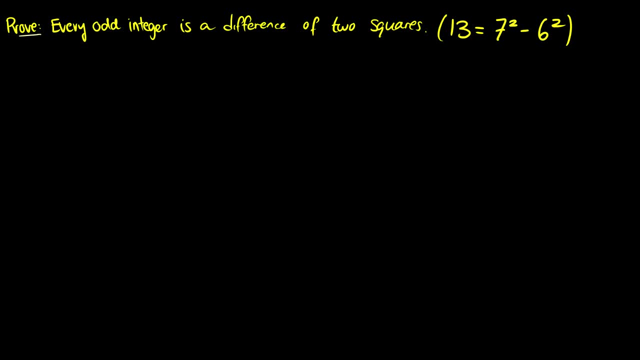 so every odd integer is a difference of two squares. so here we don't have any assumptions, we're just given a statement and we have to prove it. so every odd integer is a difference of two squares. so, for an example, 13 is equal to 7 squared minus 6 squared. let's start with a couple easy ones. 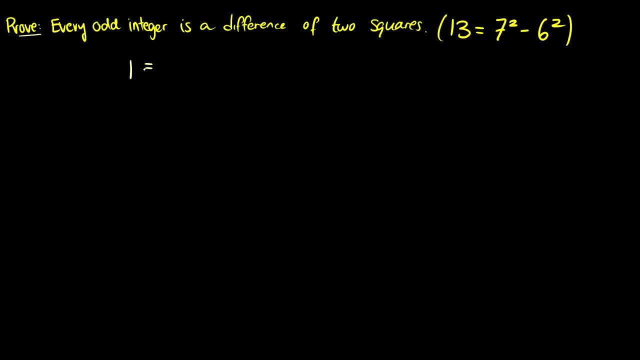 so let's take a look at one. well, this is going to be, uh, something, let's, let's think about this. if this is one, then this could be, say, one squared minus zero squared, that's equals one squared minus zero squared. what about three? well, three is going to be equal to, um, maybe two squared minus one. 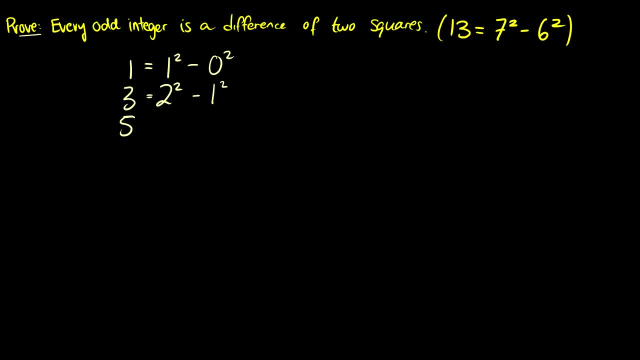 squared. and what about five? well, five could be three squared minus two squared. so of course i've done these before, so i kind of know what's going on here. so let's take a look at this one and let's kind of know what the pattern is. but it's good to check some numbers here. it's good to check these. 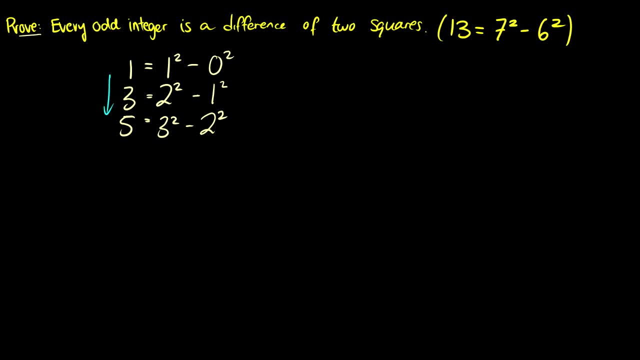 because you might see a pattern. do you see a pattern? i see a pattern. so let's take a look. how do we prove this? well, what is an odd integer? let's take the definition of an odd integer. so an odd integer comes in the form 2k plus 1 and we're saying: this is a difference of squares. 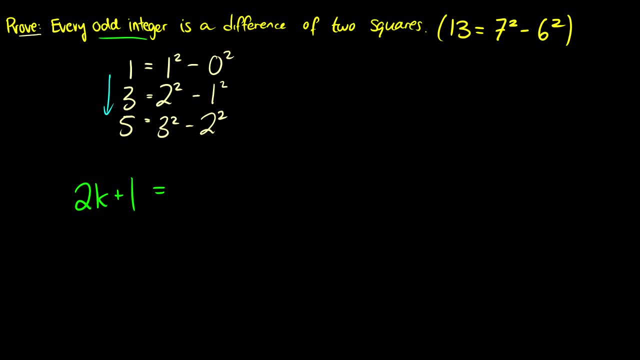 so let's take a look here. how do we write one? well, one is equal to two times zero plus one, and that's equal to one squared minus zero squared. how do we write three? well, this is two times one plus one, and this was equal to two squared minus. 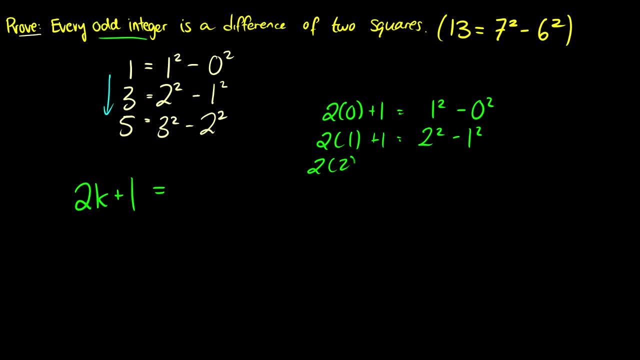 one squared. let's do one more. five is written as two times two plus one, and this is three squared minus two squared. do we see anything here that we can use? what we see? a zero here, a zero here, a one here, a one here, a two here, two here. and we're going to take a look at this one and let's 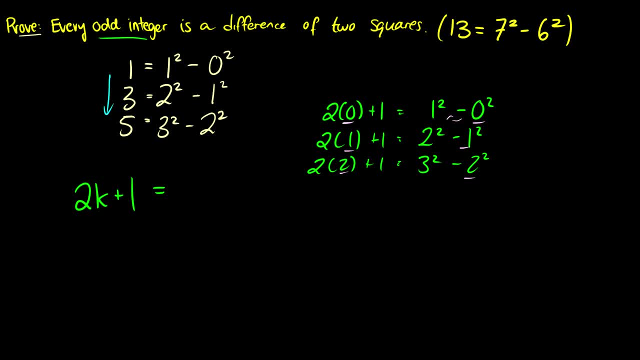 take a look at this one and then we add one. so let's assume that if our k here, so i'm going to move this down a little bit so we have room to work- okay, so this 2k plus one should be equal to k plus 1 squared minus k squared. 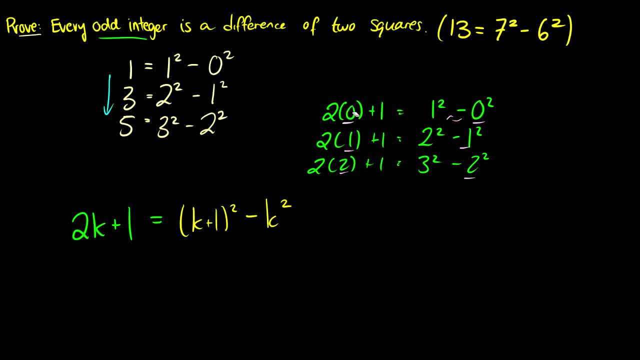 so we can take a look here. we take a look at our first example. two times zero plus one, wemani, We put a k there, then the 0 becomes a k, and then, well, what is 1?? 1 is 0 plus 1, so that's going to be k plus 1.. 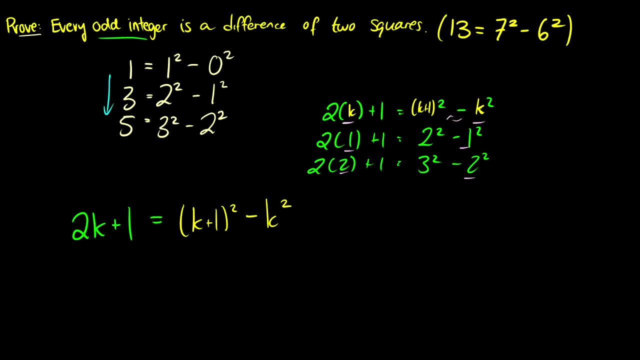 So we're going to check to see if this holds. Is this true? Okay? well, k plus 1 squared is going to be k squared plus 2k plus 1 minus k squared, So this is going to be equal to 2k plus 1.. 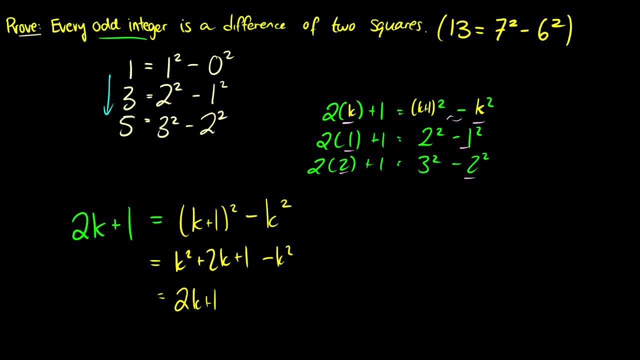 And so we've shown here that if we take the difference of two squares- k plus 1, squared minus k squared, we get 2k plus 1, which is an odd number. So every odd integer can be written as a difference of two squares: k plus 1, squared minus k. 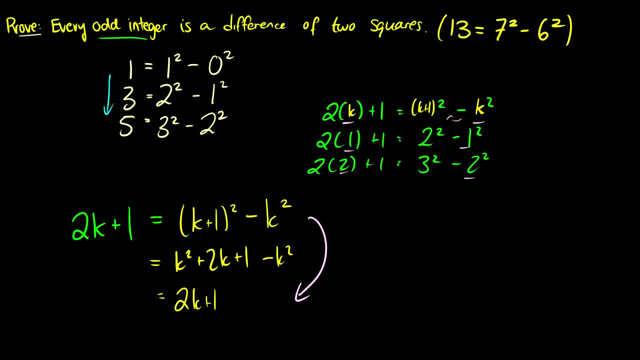 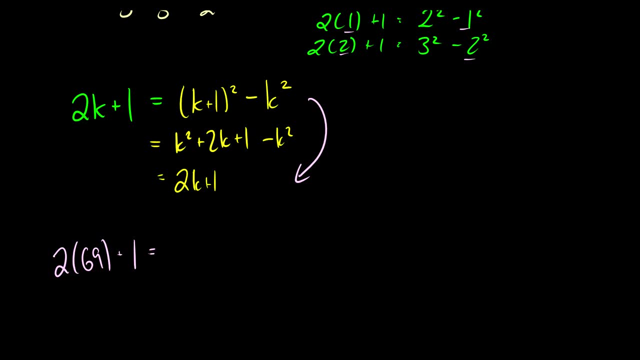 squared, So we should be able to plug this in for any value. So, for instance, let's take 2 times 69 plus 1.. This is going to be equal to well, 138 plus 1 is 139. And we're going to say that 139 is equal to 140 squared minus 139 squared. 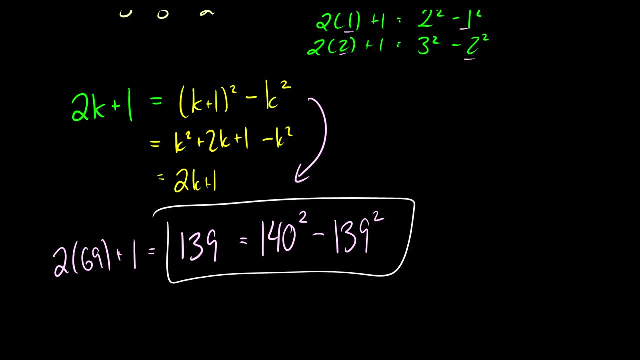 So you can check on your calculator and you're going to see that this isn't true, because this is actually 69 squared, or sorry, this is actually 70 squared minus 69 squared. This is what happens when I don't check my value of k. 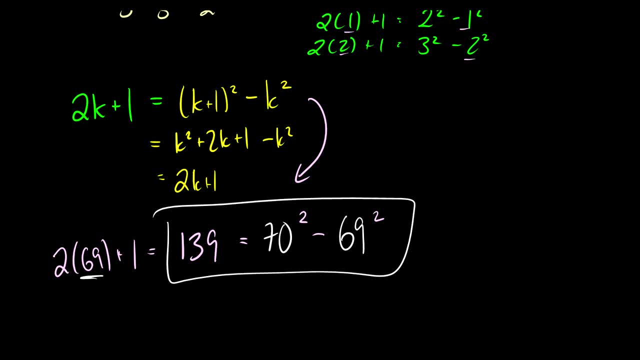 So So 139 is equal to 70 squared minus 69 squared, And you can kind of do this in your head if you want. So this is going to be 4900.. And that's going to be subtracting 461..